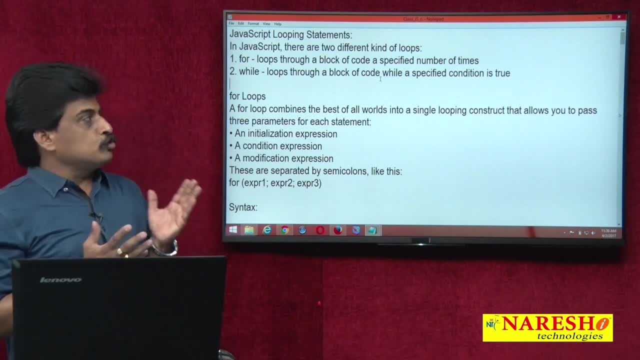 repeatedly If you come to JavaScript area for loops, same like your C programming syntax condition: initialization condition, increment or decrement. So expression 1, expression 2, expression 3.. These are the three expressions existed here. So first expression name is initialization expression. 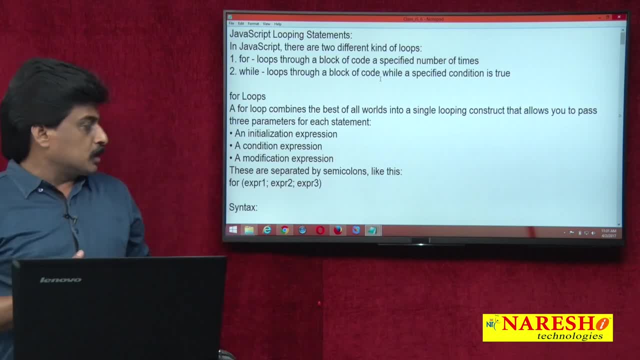 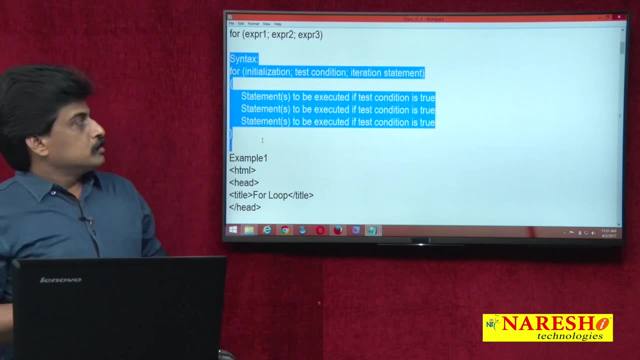 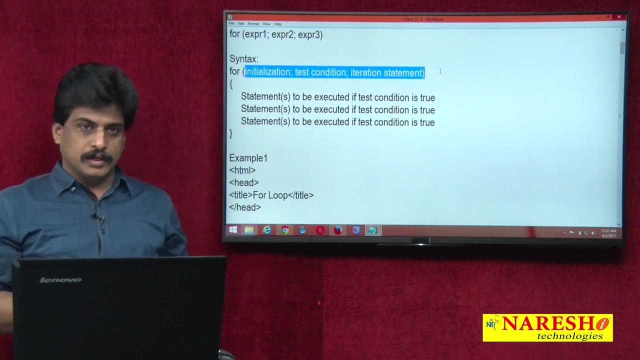 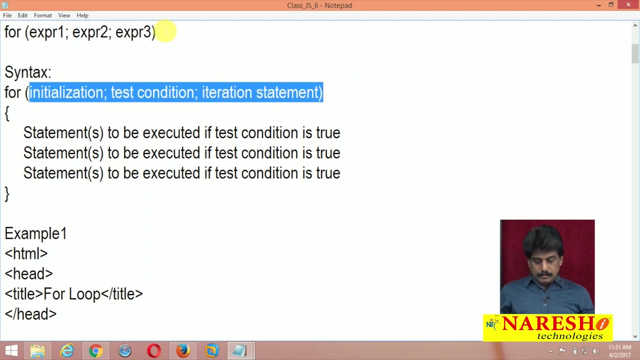 Second, one is condition expression. Third, one is modification expression. Now the syntax. wise just observe. So this is the syntax. What exactly we are implementing in C language? The same syntactical we can try to implement in our JavaScript. Right the first. 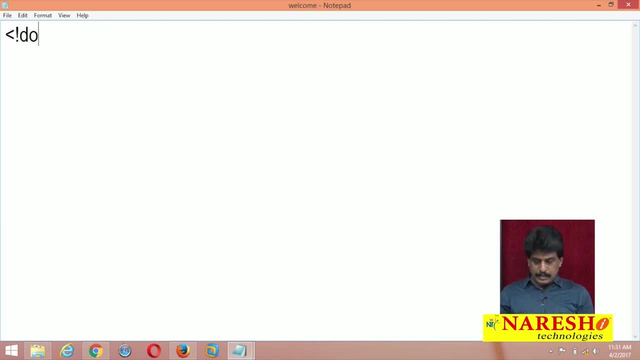 example, using for loop doc type general, I am writing Simply the structure I implemented and I am moving inside, For I is equal to, I less than or equal to document dot. write plus concordination You want to display. next line means add: write br tag. 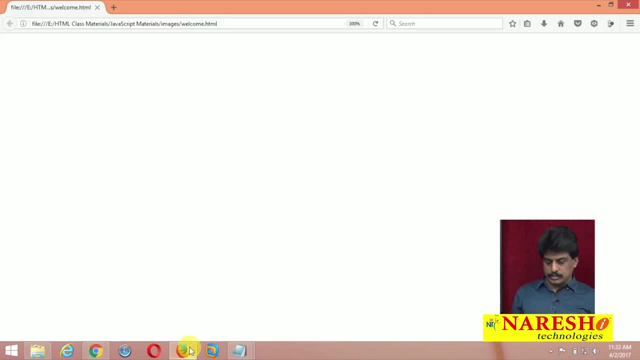 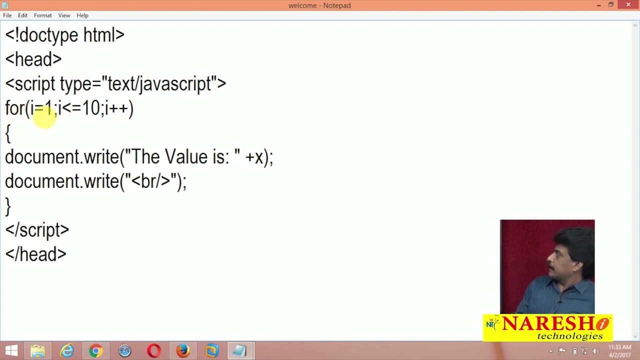 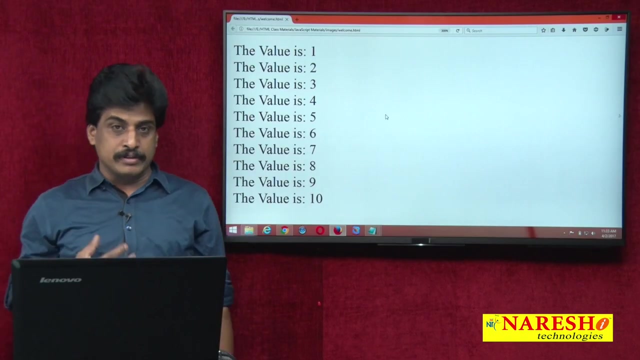 refresh on your web browser. Come back Document dot. write the value: is x actually used variable? is i Very good? Come to know it that Intentionally? some examples: I am making Small, small mistakes and recovery. Simple one: I? u declared x. you are displaying How output will come, So I modified that. 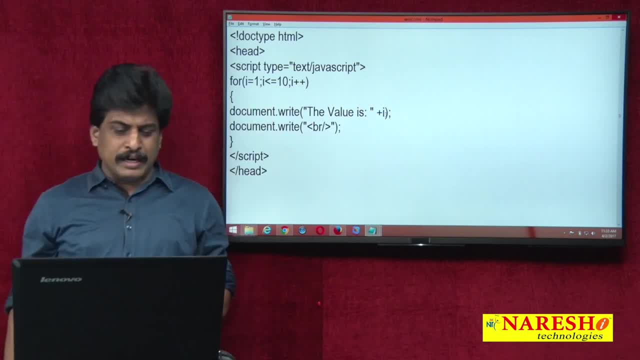 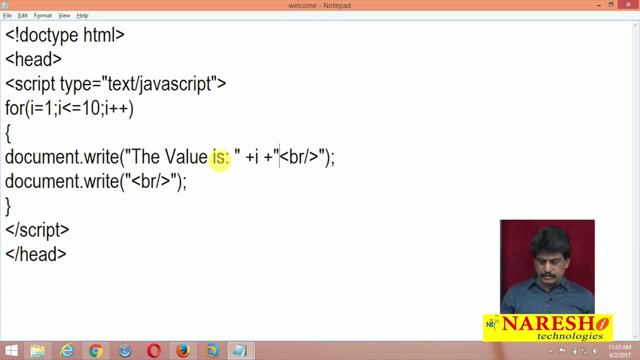 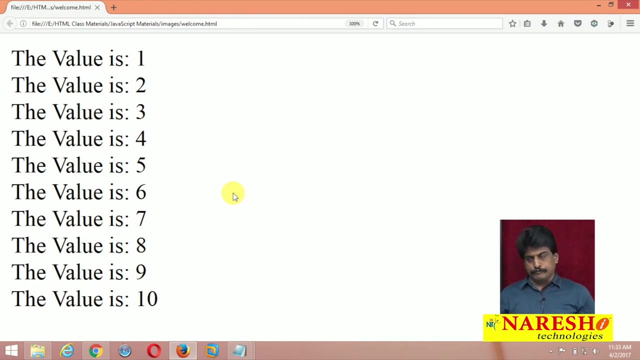 I and I So perfectly, Why we are writing again. break another line. Just, you can go to Concordination and it should be within the quotation Write better example: Refresh: Perfectly executed. So far better, simple, easy to answer. 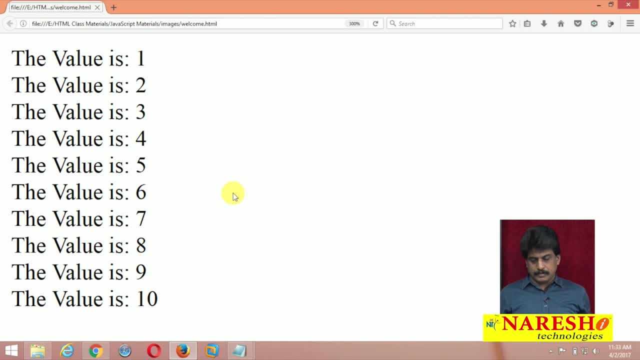 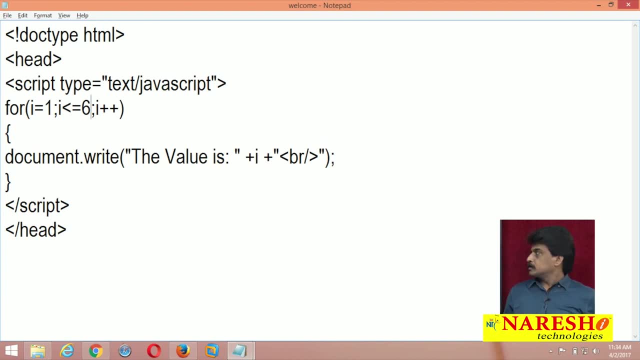 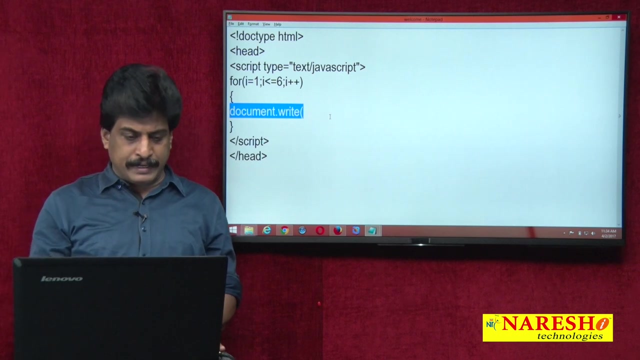 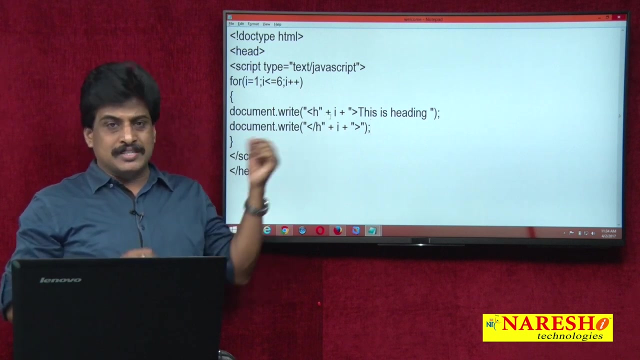 Already. see programming syntax. is there easy? Come back. And now I am implementing here html headings 1 to 6: headings i is initial value 1, so h1.. I need to write that documentwrite. so whatever I am implementing here, simply h i concordination. 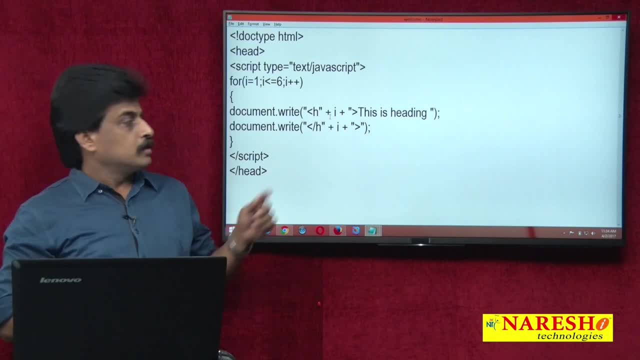 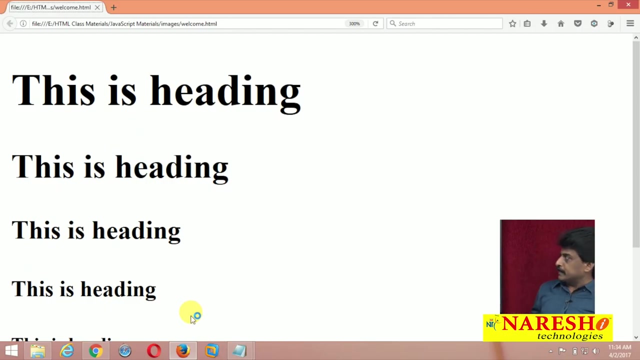 So this concordination is providing to us initial value: 1, h1, plus this heading is: And again you need to close. So like that, first time, 1, 2,, 3, 4, like that- Now I am going to run it perfectly- get executed. 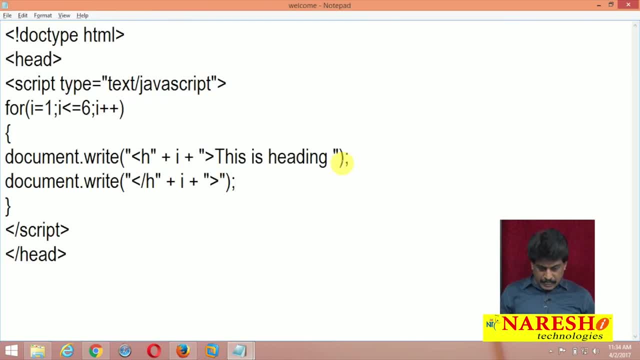 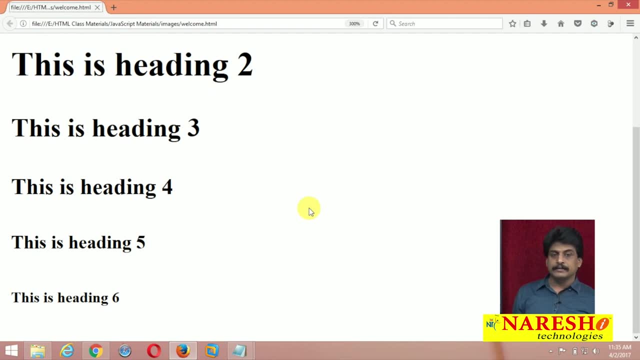 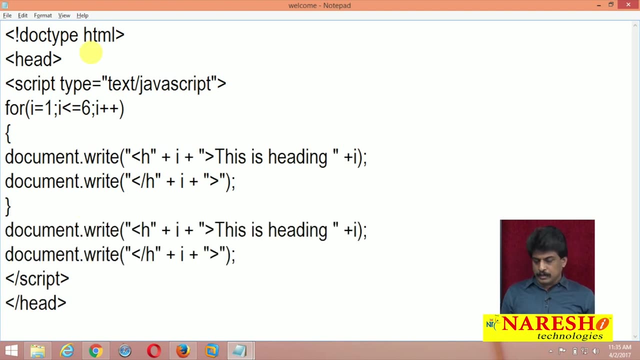 This is heading 1,, 2, 3.. You want to see that plus i. You can apply, you can view the things: one heading second, heading third, heading fourth, like that example. I am going to take this value and I am going to come out of the block and I made for. 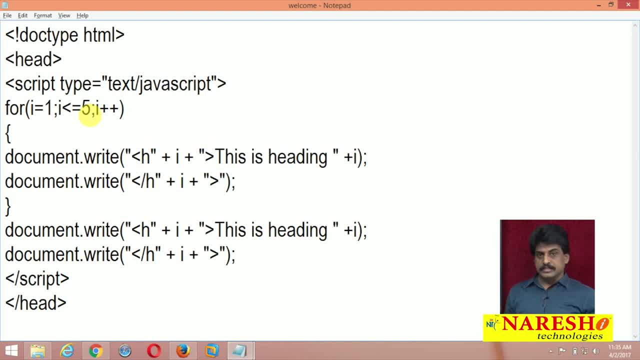 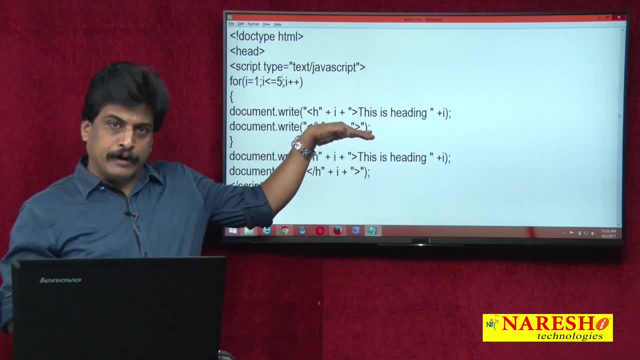 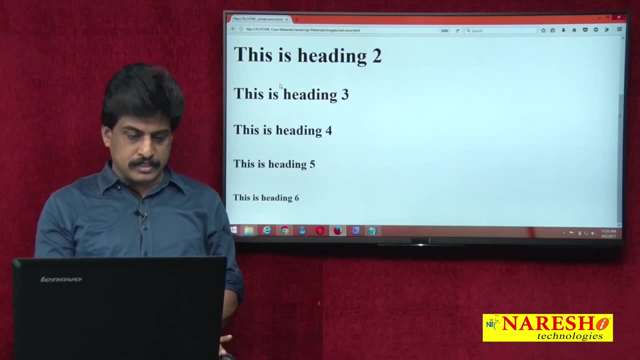 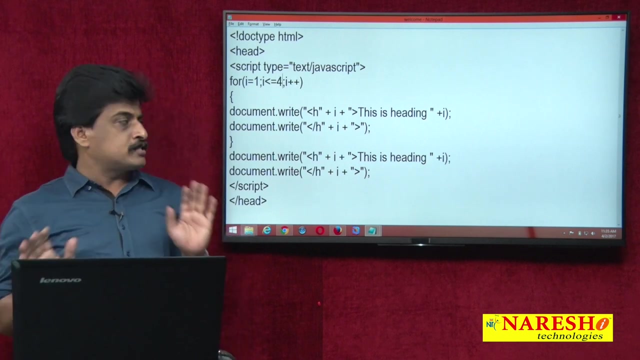 example, 5.. So what is the output of this Same output previously. like that, any changes. So this block will be displayed up to 5.. When it is 6, the condition falls. then it is coming out. So same previous output. there is nothing changes. For example, I am coming to here 4, then I set the. 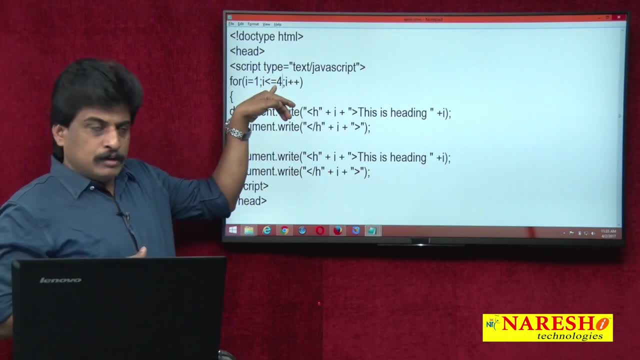 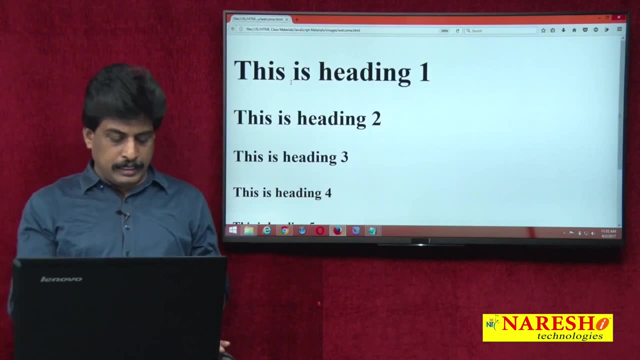 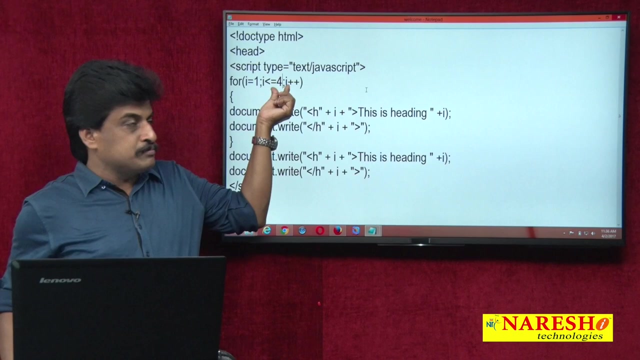 same example: When condition 5 falls, when 5 it is coming out. So up to 4, this block will be displayed, only 5, this block. So here, only up to h5, no 6.. So understand this simple logic. what I am saying is: 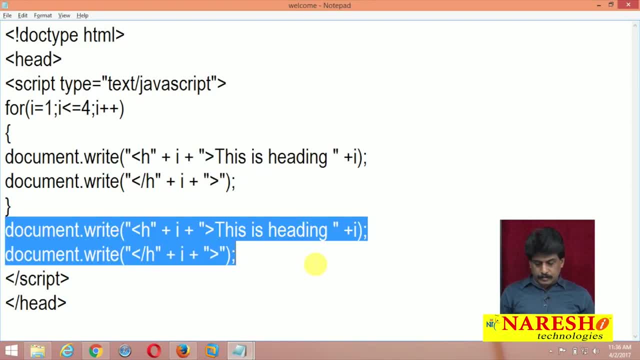 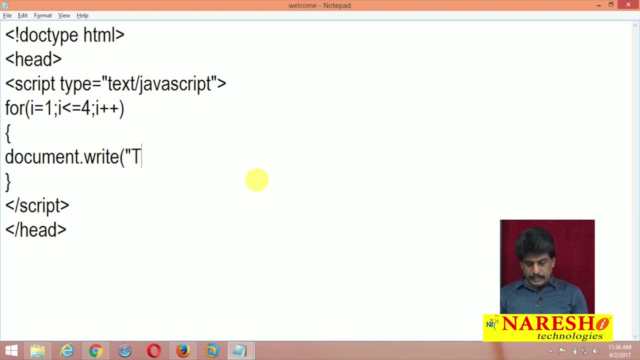 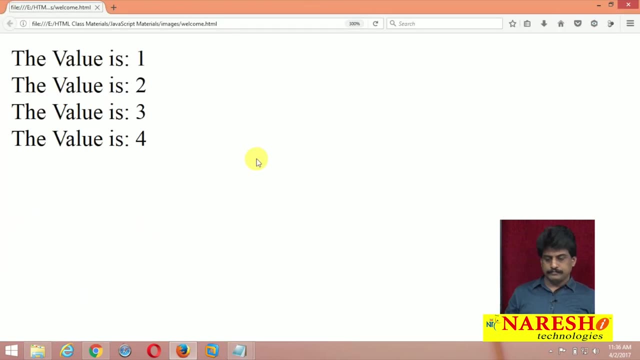 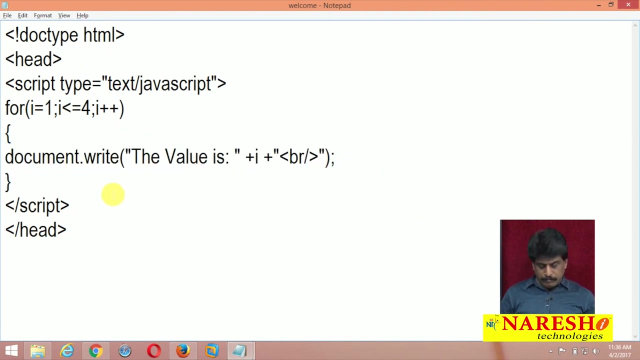 here, Just you can come back. We will go to previous example. simply Document dot. write the value is break. quotation, observe 4.. Good, come back Now. for example, out of the loop, I want to display the value. So then what will be? 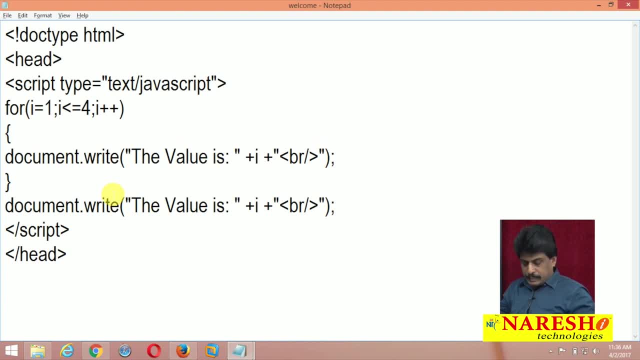 displayed When 5 the condition falls, So that 5 available here. So now it displays 1, 2, 5.. Understand very simply that whenever condition falls, the value available out of the loop. If you are displaying the same value again, still the same value available, What that one, 5, 2 times This is. 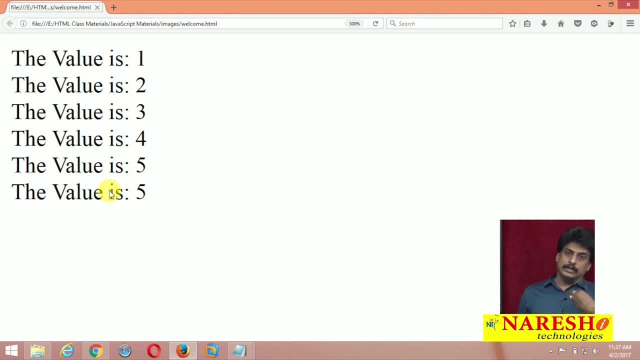 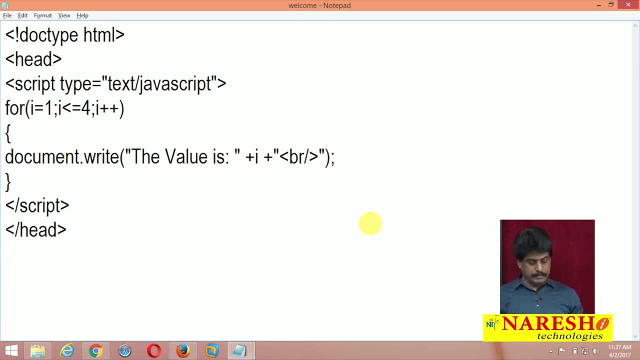 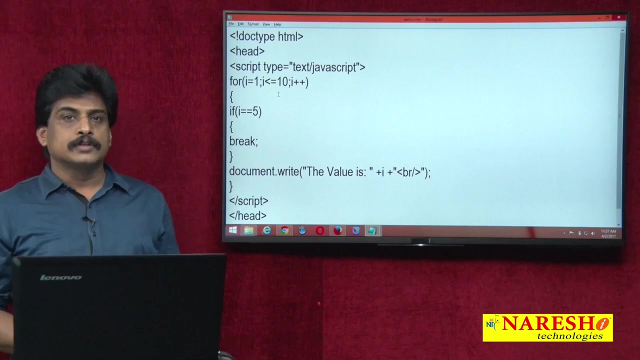 the for loop, what the exact out of the loop. also Now come down Here: break and continue. 2 statements available. Go to for i. is i less than r Equal to 10.. I am writing if i equal to 5.. I said break. That's all. So what is the output of the? 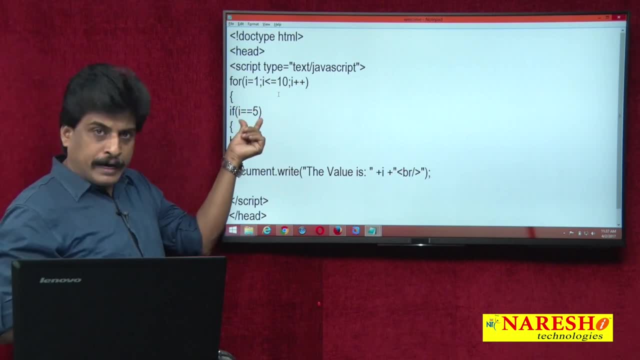 program Actually 1 to 10 numbers, But you said when 5 you should break. Break means it terminates the loop. When terminates the loop, then 5.. So what is output of the program 1 to 4.. Correct. 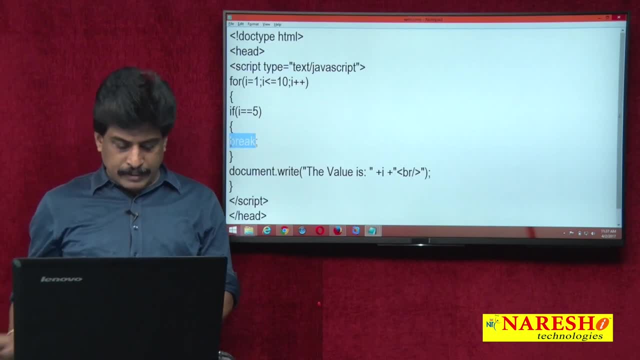 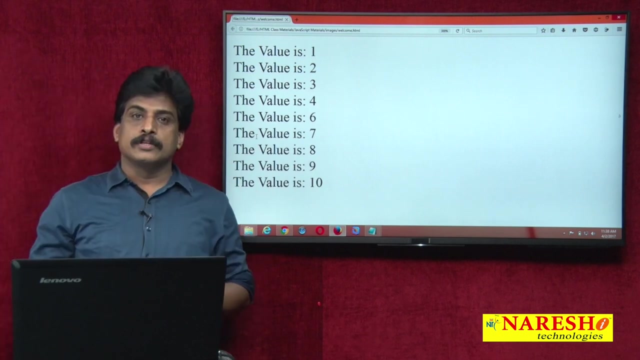 Right, Come to next one: Continue. And we are taking that Right. This is a continue, Except the given condition means except a 5, 1 to 4 and 6 to 10 values will be displayed. So it is terminating only the condition value Remaining. 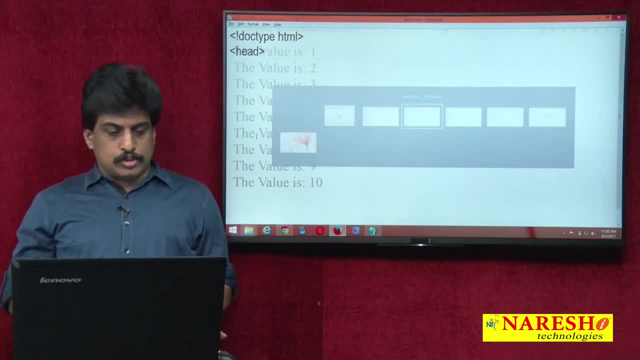 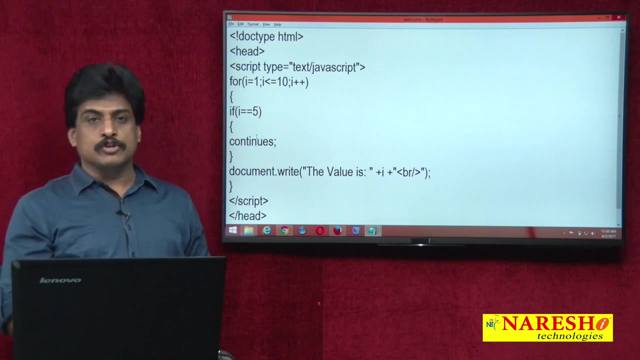 values as usual displayed. So this is about a simple for loop. Little inside we can observe, That is only while while same like for, but there is a small difference. it executes block of statements repeatedly Until the given condition. false means n times It is running. 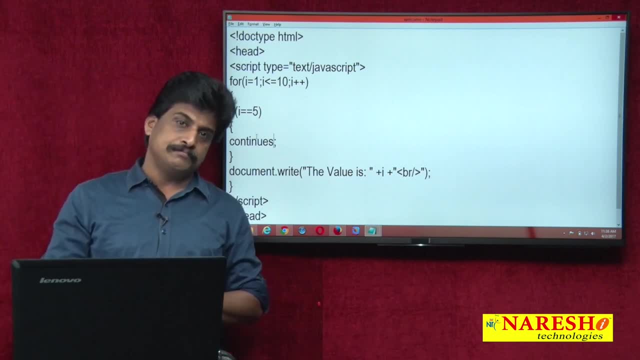 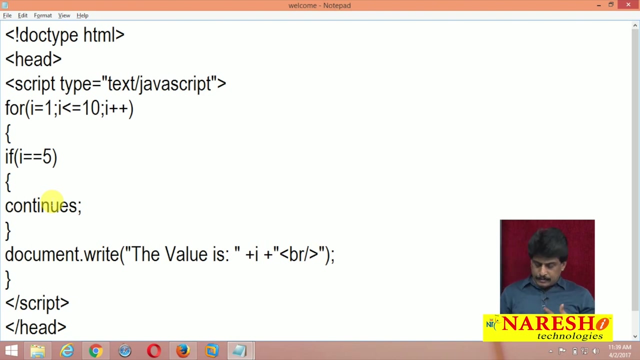 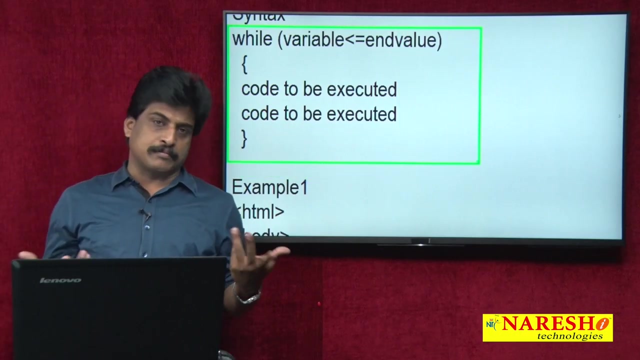 Here min and a Max values are not compulsory. That is a minimum iterations, Maximum iterations. If you are observing in java it while syntax while condition do statements done generally, but here while condition statements will observe that while condition statements in some scripting languages do done also available. 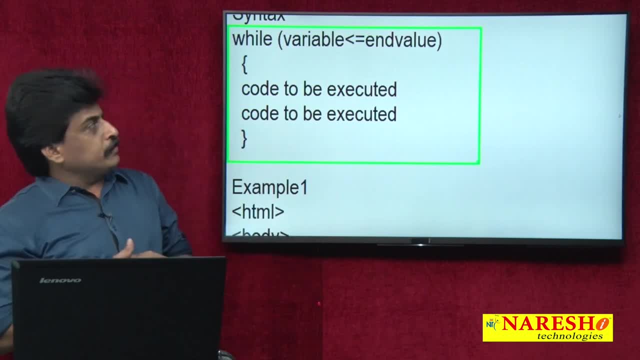 here only while condition statements. ok, now we can try to write: while condition i less than or equal to 10, i am declaring i is equal to 1 and while already i said 10. after that one document dot write the value is i, i++, otherwise how it will increment if you write. 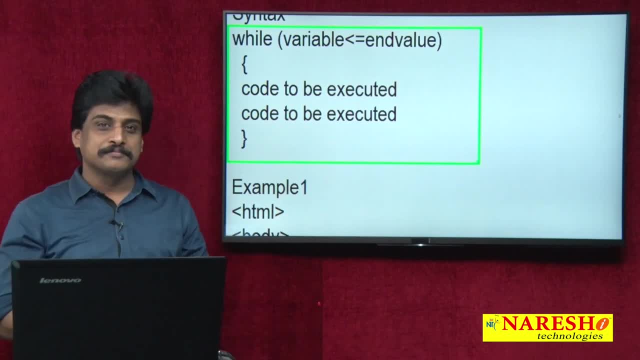 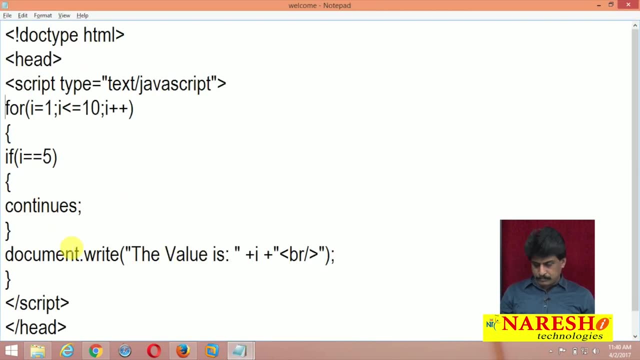 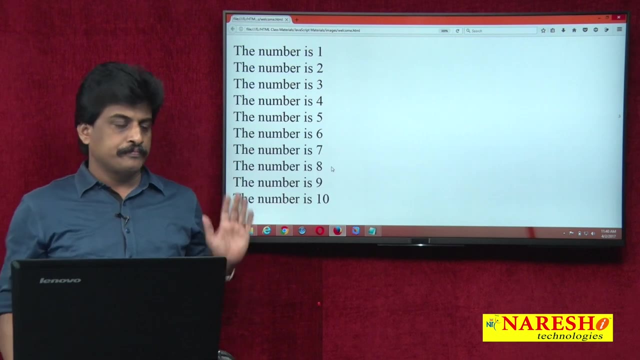 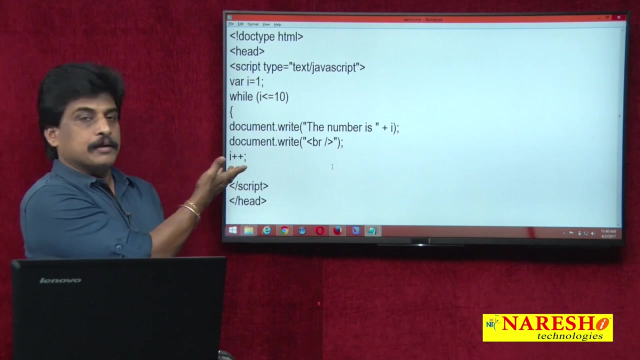 document dot, write i. it will display only one value, 10 times so i++. then you need to close without any late. simply we will write that: remove the statements. write so: i implemented, completed. So just you can refresh same output and observe initialization condition increment. so then. 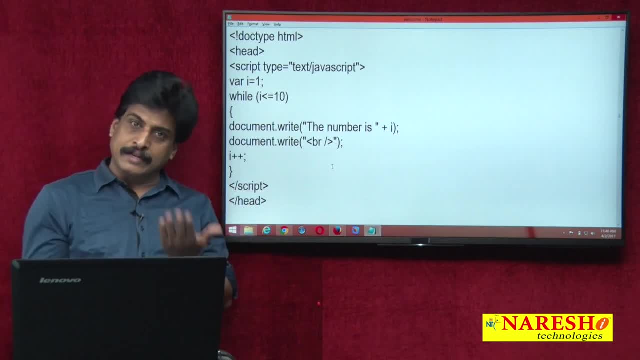 previous programs, whatever implemented. i can do with the while. you can try it. that next do while it executes. block of statements n plus 1 times. n plus 1 times means you people are understanding this: first statements executed, next condition executed. that is the reason i said n plus 1 times it executed. 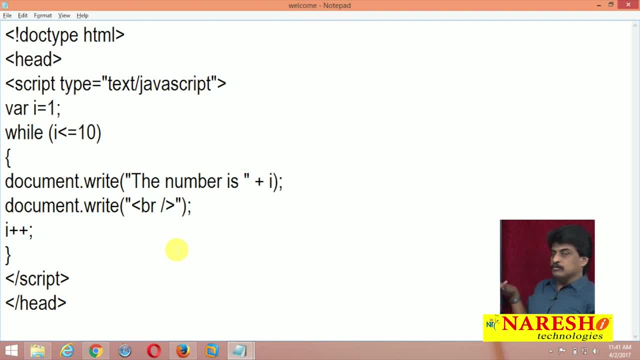 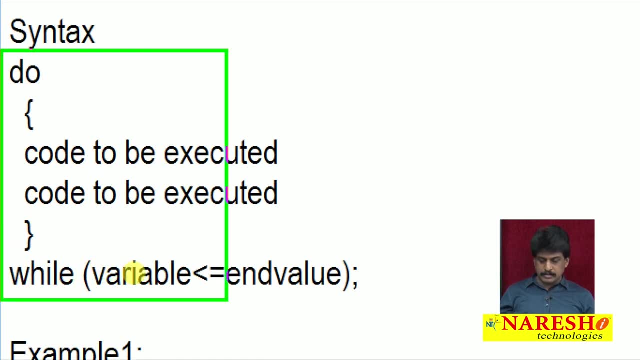 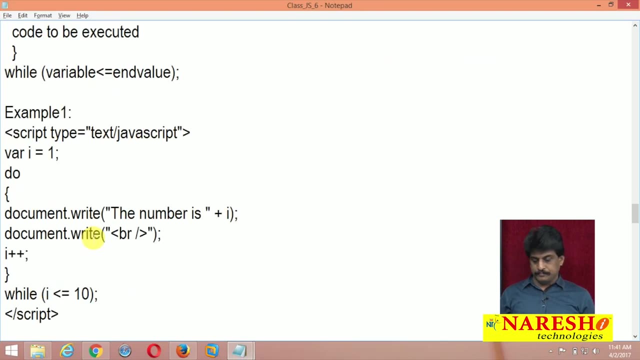 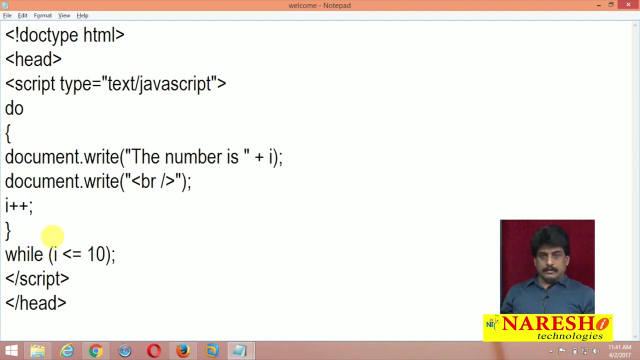 The same syntax, but while condition will be displayed last. first syntax. we can observe the syntax of do while, do statements while condition. write one simple example. same previous example. i am changing to this. yes, same previous example. time while condition. i wrote here just that, while i wrote last. 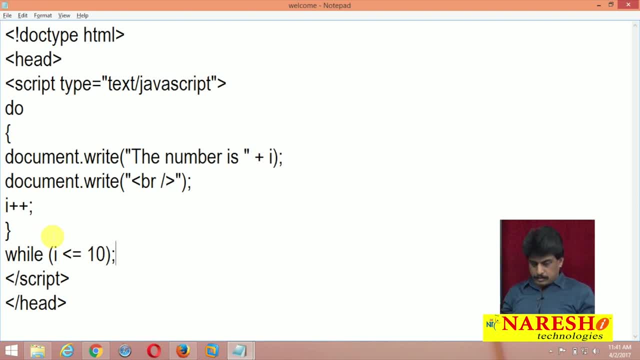 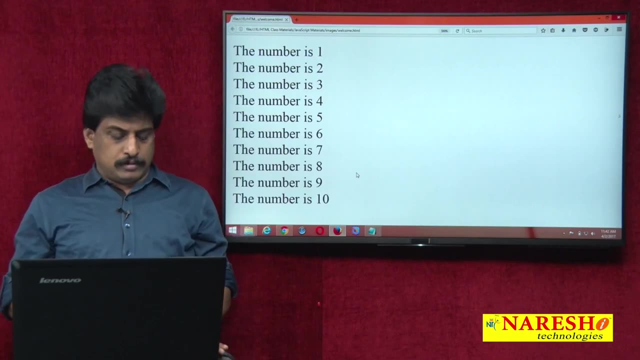 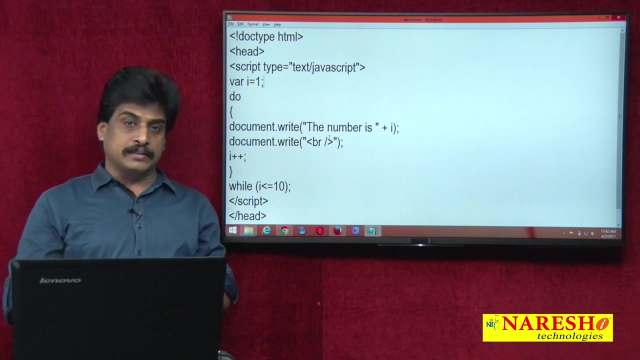 Ok, Last semicolon refresh and you can run it once you come back. while, condition do, statements i++ perfectly displayed right now. we can see: while, do, while, very simple logical programs. while is nothing but n times do, while n plus 1 times for with with break. 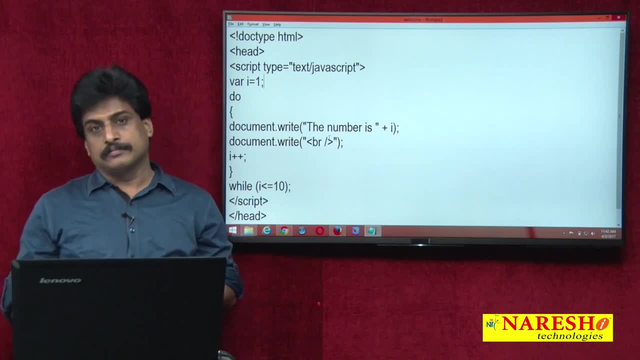 As well as continue. so now, one by one, we can try to understand these looping controls. after these simple looping controls, actually we need to implement in the project level how we are going to be the purpose. at the last video session time, i will show you one application.